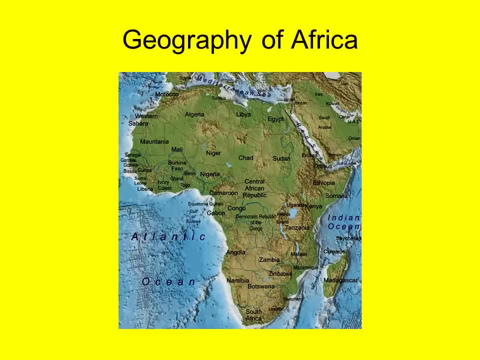 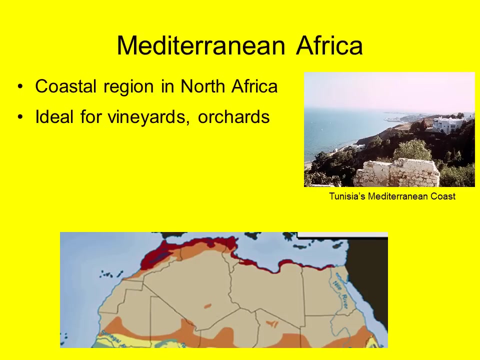 In this lecture we'll be taking a look at the geography of Africa, some of the major landforms, the waterways of the continent and how they have affected the history and culture of African civilizations. First, we'll take a look at a region we're going to call Mediterranean Africa, along the Mediterranean coast. 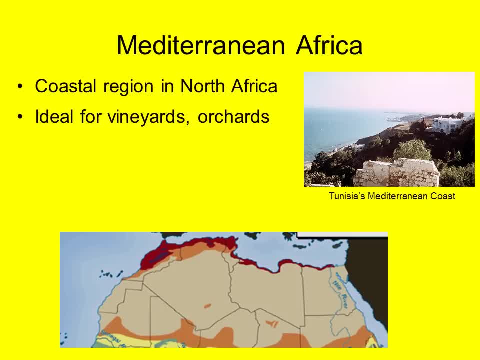 The features of this region share a lot of similarities to southern Europe and Mediterranean. Africa is prominently featured in European history. The Greeks, the Romans colonized this region and, going further back, so did the Phoenicians. The area is known for mild rainwater. 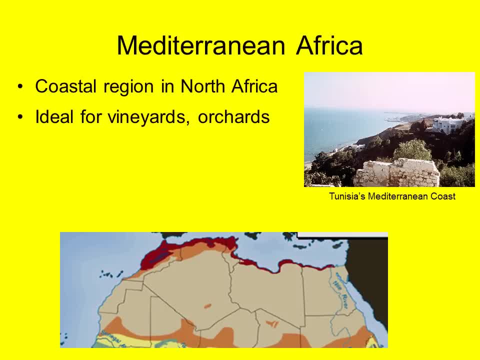 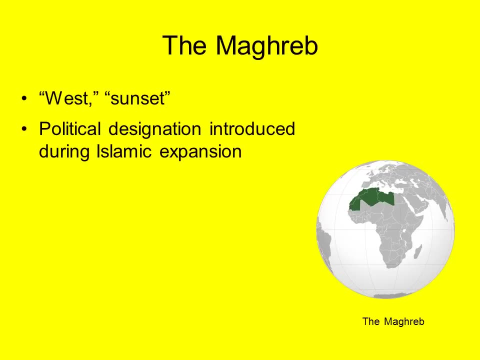 This region is known for its rainy winters and hot, dry summers, very much like southern Italy, southern Spain and Greece in terms of climate. The Maghreb is typically defined as most of the region of northwest Africa west of the nation of Egypt, the modern nation of Egypt. 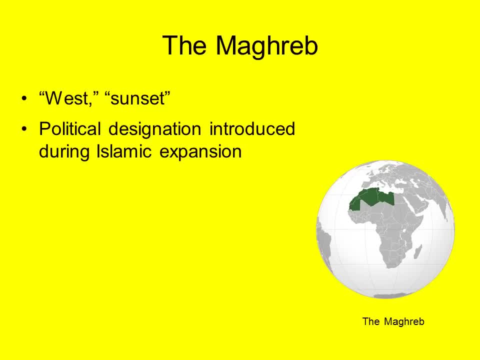 The word, as you can see on the slide, translates as west or sunset. So it's the idea. So, if you were thinking, in the Arabic language, this is a political term for the most part to describe a region. so we're not going to discuss specific climatological associations here, because they do vary. 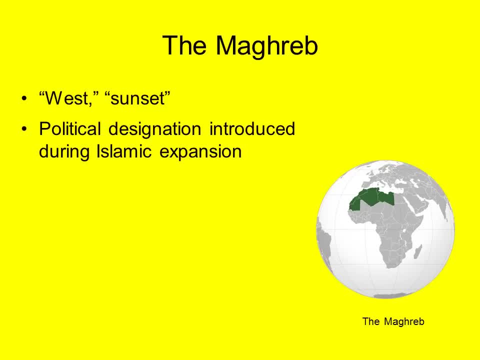 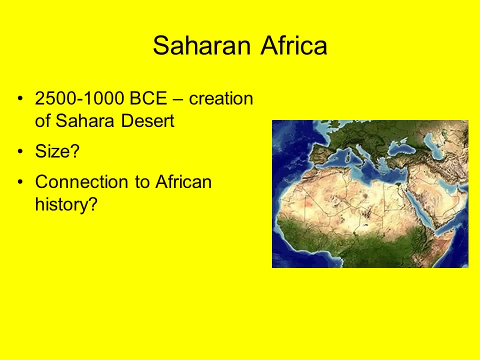 In the modern world, this would be the countries of Morocco, Algeria, Tunisia, Libya and Mauritania, plus the territory of western Sahara. The Sahara itself, as most of you know already, is a desert. It's the Arabic word for desert. 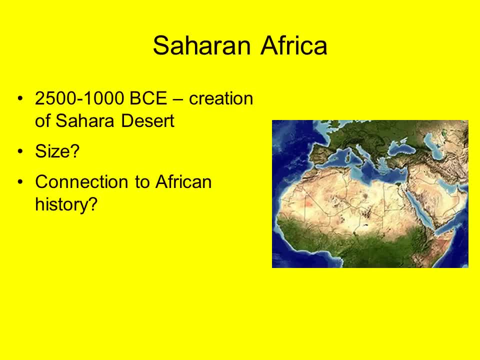 It also carries connotations of a desert sea, So we'll get to that in a second. It's about the size of the United States: 3.3 million square miles or so. It is increasing in size. right now, Temperatures can reach as high as 130 degrees Fahrenheit during the day, and below freezing at night. 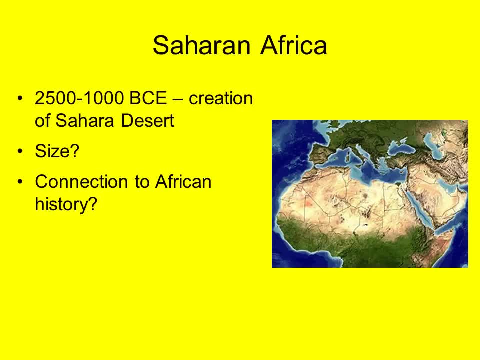 It is sparsely populated, but about 2.5 million people live in the Sahara and it's a variety of ecosystems, not just sand. You have mountainous regions like the Atlas Mountains. At one point, the Sahara was a marshy region about 6,000 years ago. 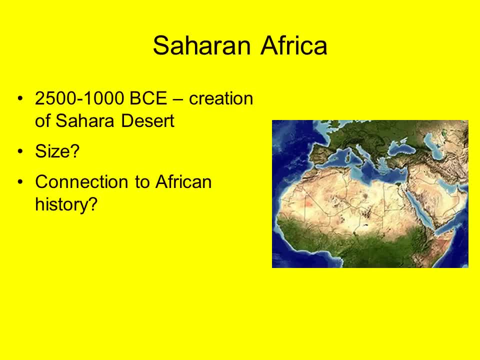 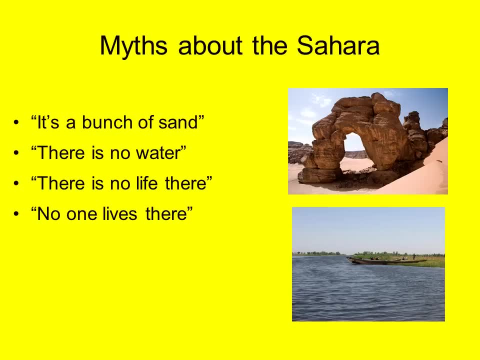 Since that time, it has dried up, of course, and it is currently still expanding. There are a number of myths associated with the Sahara. As we indicated in the previous slide, it's much more than just sand. There are significant water deposits in various places, although, because it's a desert, of course, these are few and far between. 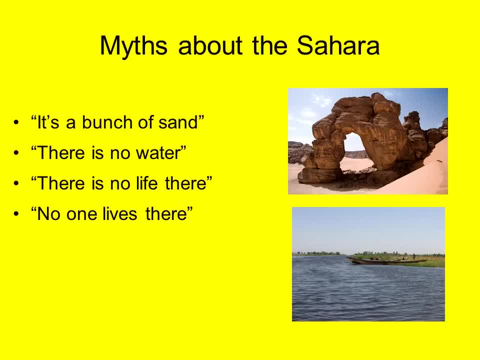 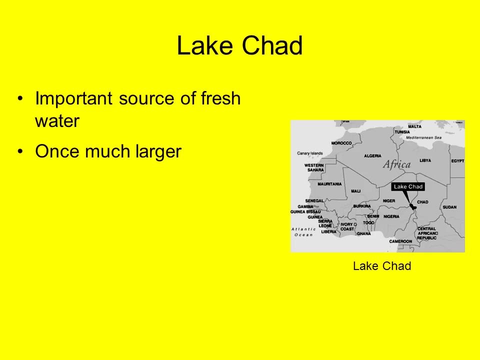 Quite a variety of life manages to exist and even thrive in the Sahara And, again, as we indicated in the previous slide, 2.5 million people call the Sahara Desert their home. Lake Chad is a freshwater lake in the Sahara River. It's a relatively shallow lake, about 35 feet at its maximum depth. 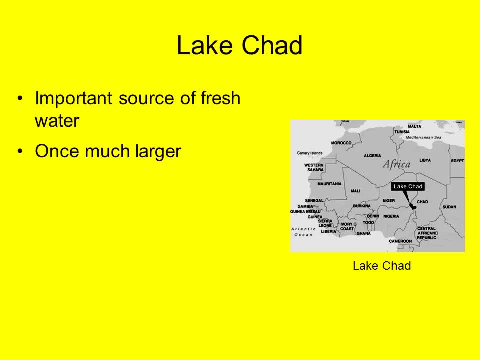 The size greatly varies seasonally, with the flooding of wetland areas. There has been a significant amount of shrinkage of the lake due to climate change, irrigation and inefficient dams. It is also, interestingly, a home to many floating islands. 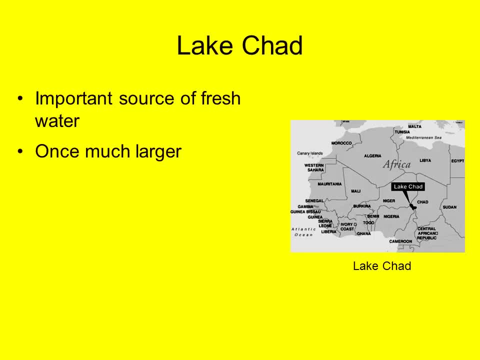 These are, in some cases, man-made structures and in some cases, artificial structures, But topsoil has been added to plants that float on the water And many people in the Lake Chad region actually live on some of these floating islands. About 20 million people in Africa depend today on water from this lake. 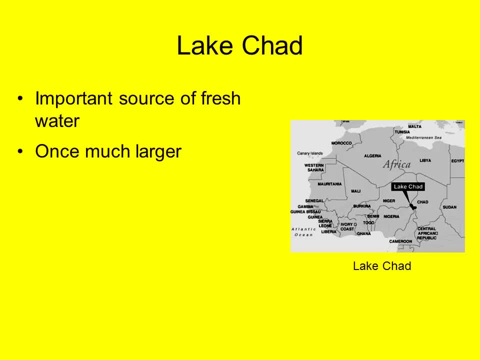 But again, about 90% of the lake has disappeared since the 1960s And the future is not that good for the lake. But perhaps water management policies enacted by the nations of Chad, Nigeria and Niger will be successful in restoring the lake. 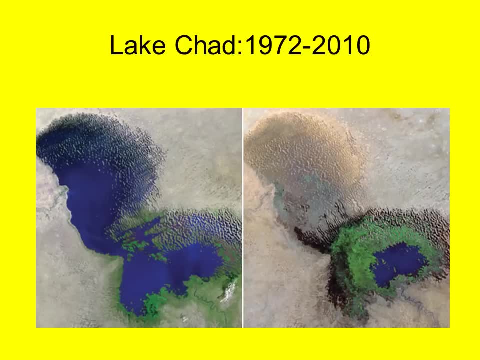 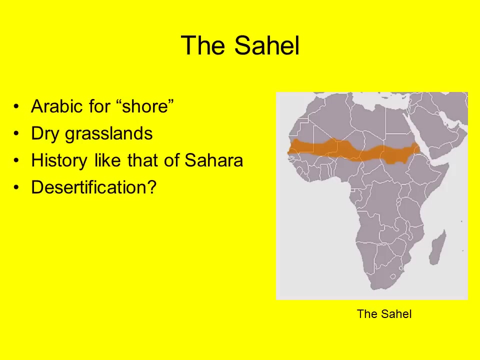 This slide shows aerial photographs indicating the amount of shrinkage of Lake Chad. You can see it's very significant And portions of the lake bed have reverted to desert. The Sahel is a region south of the Sahara. It translates from the Arabic as shore. 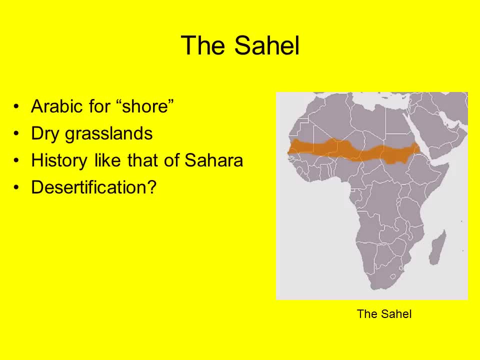 So if you're thinking of the Sahara as a giant sea, a sea of sand, the Sahel would be the shore of the sea. It's about 3,400 miles long, up to 500 miles wide, And it too, like the Sahara, is still expanding. 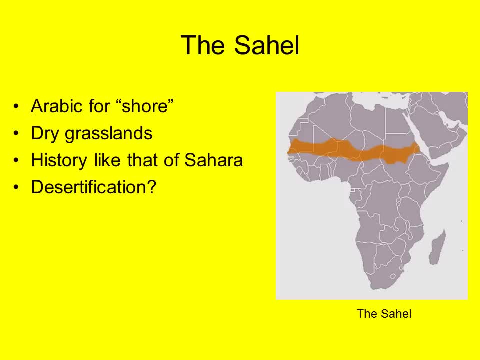 Some of the most advanced African civilizations emerged here in this region, including the Trans-Saharan trade routes that emerged. Its history is much like that of the Sahara. Its geological, climatological history once had a great deal more water and life forms. And as the Sahara increases, the Sahel also increases to the south and to the east. 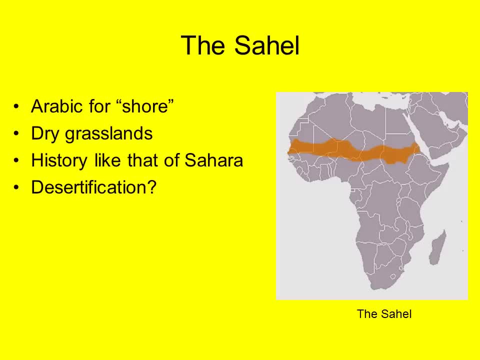 This is a region known for transhumance. Trans means activity, trans from the Latin meaning across and humus meaning ground. So across ground, a lot of trade routes and herding, Over-farming, over-grazing and over-population of marginal lands, plus natural soil erosion. 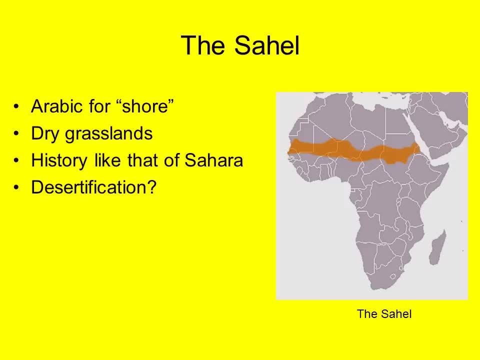 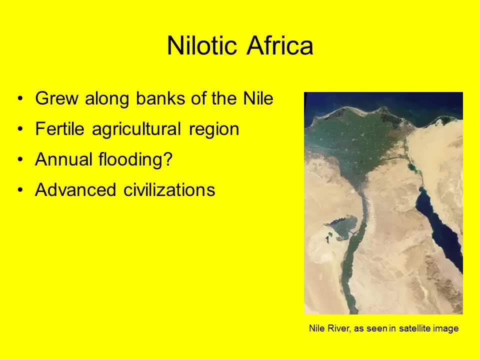 has caused serious desertification in the region. Nihilotic Africa refers to the regions in and around, immediately around, the Nile River. It's an extremely fertile agricultural region. The Nile River, if you weren't aware, traditionally floods almost like clockwork. 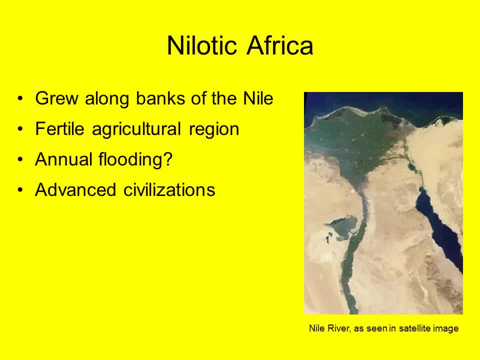 And the annual flooding brings with it nutrients and silt from upstream. This has changed somewhat in the modern era, as dams have been built on the Nile to control the flooding, So this has meant less disruption for people to live along the lower reaches of the Nile as it approaches the Mediterranean. 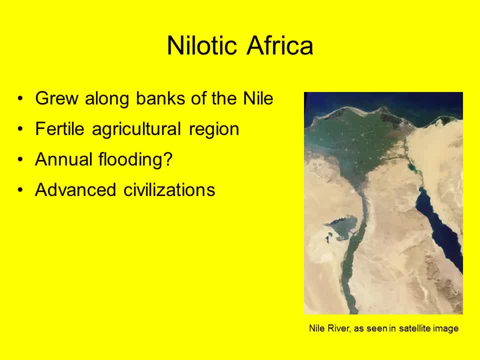 But at the same time that has had some negative effects on the fertility of the soil in the region, So kind of a double-edged sword in terms of annual flooding. Many advanced civilizations emerged here. We talked earlier in the course about the importance of the Nile in Egyptian culture. 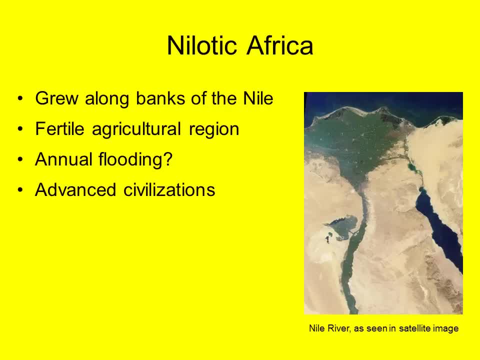 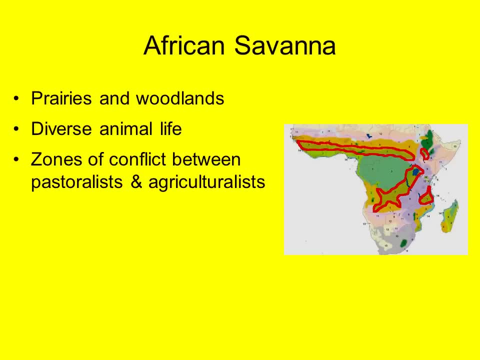 And in this segment of the course, as we talk about Africa, we'll talk about some of the other kingdoms that called the Nile home. The African Savannah region is south of the Sahel. It is perhaps culturally familiar to many Americans because it's prominently featured in programs like National Geographic or pop culture films such as The Lion King. 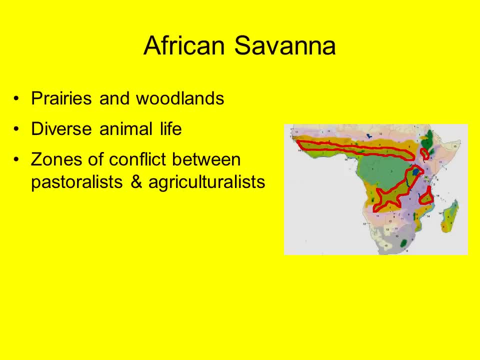 One of the reasons we, as Americans or Westerners, are fascinated with the Savannah is because of some of the interesting life forms that can be found there: Animals like the zebra, the wildebeest, the water buffalo, giraffe, the impala- some of these almost iconic animals called the Savannah region home. 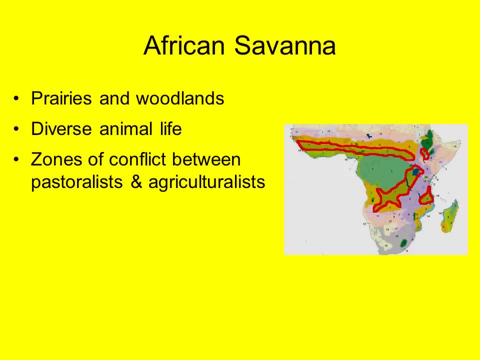 Overgrazing, animal poaching and soil erosion have been major problems in the last few decades. This has also been an area in which there's been almost constant conflict Between pastoralists. those are people who herd animals such as sheep, goats and cattle, especially cattle. 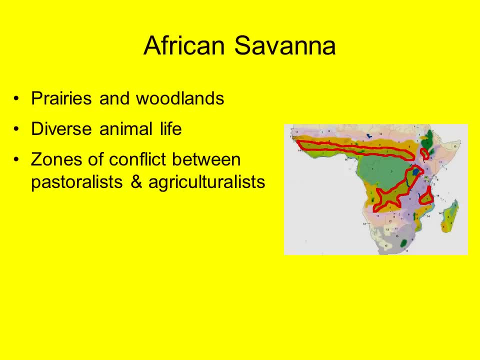 And agriculturalists- settled agriculturalists who grow crops, So herding animals of course like to eat green plants and agriculturalists like to grow green plants. So you can see where there's some contention over land use and rights to use land. 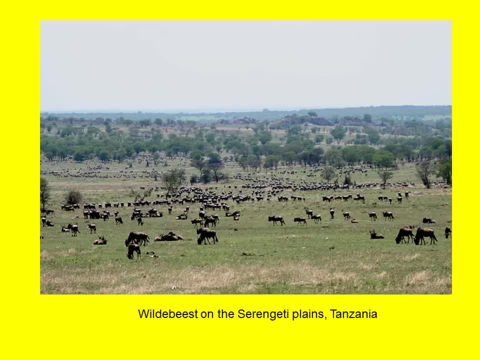 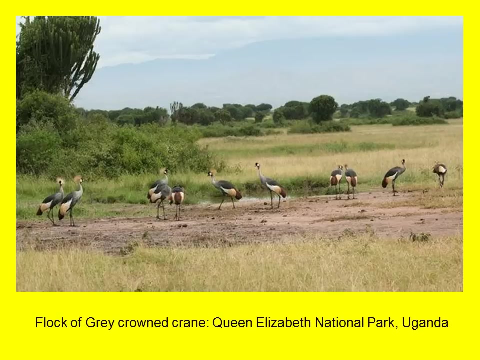 This is an image of an annual migration on the Serengeti Plains in Tanzania of the wildebeest. They travel thousands of miles each year back and forth across the Serengeti Plains. Here we have a gray-crowned crane in Uganda, also part of the Savannah region. 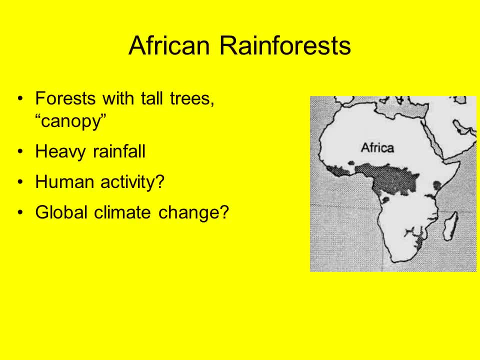 The rainforest region is home to half the savannah. It's the continent's animal species. Many hunter-gatherer societies emerged here due to the immense plant and animal diversity, And in a region where there is such a wide variety of life forms, both plant and animal. 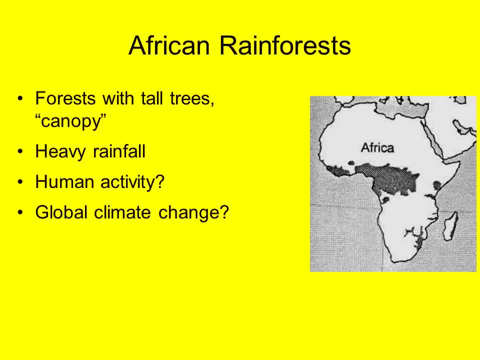 it's much easier to be a hunter-gatherer as opposed to say, in the Sahel and Savannah, where life is a bit more sparse. In the Sahel region, road construction slash and burn farming have wiped out about 90% of West Africa's rainforests. 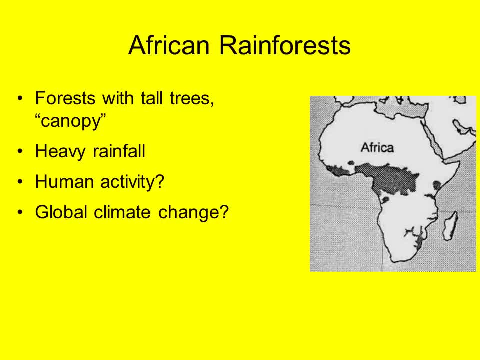 And poaching and illegal logging are major problems. There has been some concern- and again, climatology is a newer science, but some concern- about the connection between global climate change and the deforestation of the rainforest regions. Research is still ongoing on this, but in all likelihood there's probably some connection. 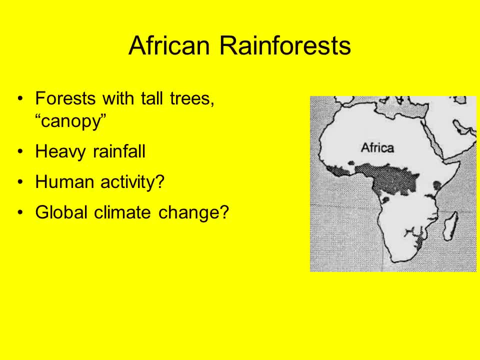 between climatological events that are happening around the world and the shrinking of the rainforest. To what extent this is cyclical? to what extent is this caused by humans? of course, is the real debate, But there's no question that the amount of rainforest region is rapidly shrinking in Africa. 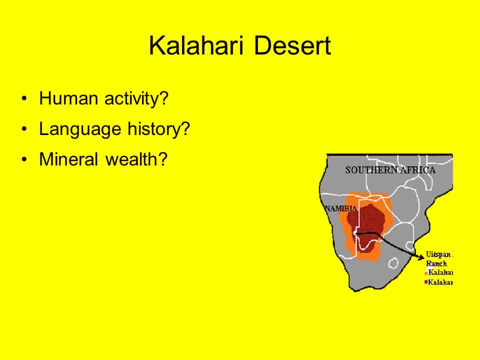 Moving further south, we are looking now at the Kalahari Desert region. In some places it's not quite a true desert, it's more like a very dry savanna. So if you're looking at the map, the orange region would be more of the very dry savanna region. 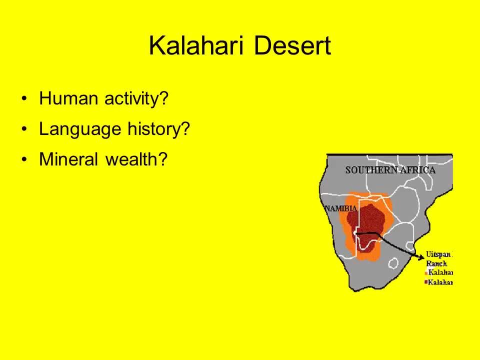 and the red would be more of the true desert region. A significant amount of pastoralism, especially cattle herding, occurs in the Kalahari Basin. There's vast mineral wealth in the region. Items such as diamonds, tin, copper and gold can be found- deposits of these there. 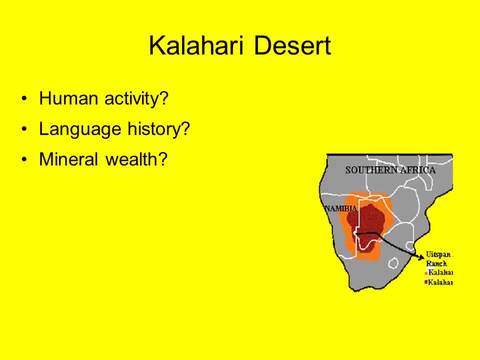 And of course, the extraction and the competition for the rights to extract these minerals has led to significant conflict, especially in the recent century or so most recent century. Lake Magadigadi once covered most of the Kalahari, So this was once a giant lake thousands of years ago in Africa. 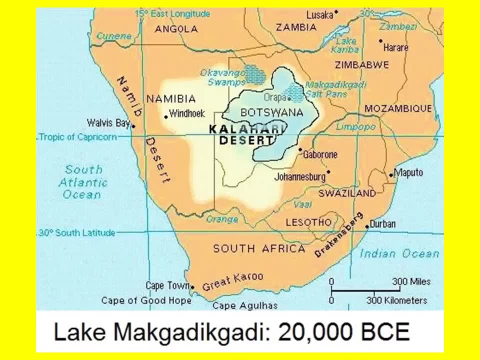 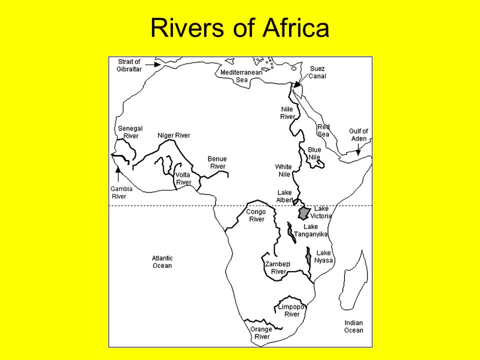 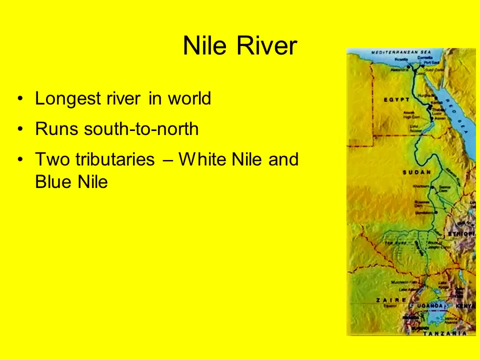 Here's a map of the basin of what was once Lake Magadigadi, 20,000 years ago. Let's turn next and briefly discuss some of the major rivers of Africa. The Nile River, a little over 4,000 miles in length, is the longest river in the world. 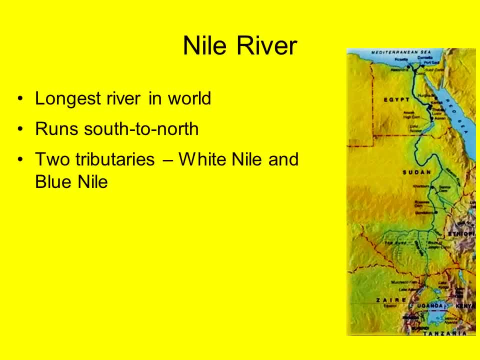 It has a drainage basin in which about 10% of the African land mass empties. The Nile itself has been a source of what I call exploration obsession for Europeans. They always as soon as they, as soon as Europeans- arrived in Africa. 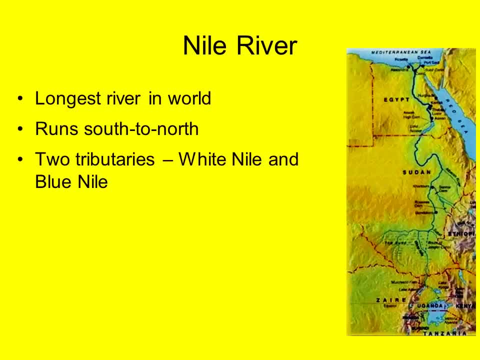 in northern Africa were intensely curious to find out where it starts. For a long time, Europeans believed that the Nile and the Congo were one river and that they sort of cut right through Africa. The White Nile has as its source the Lake Victoria watershed. 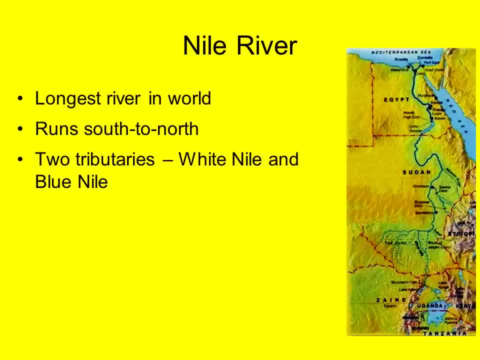 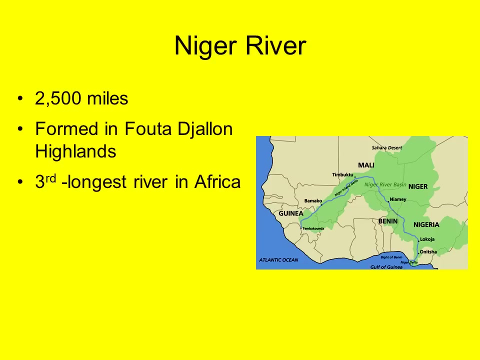 The Blue Nile- those are the two main tributaries- has its source in the Ethiopian highlands And, as we indicated earlier, yearly floods bring new silt and sediment for very productive soil in and around the Nile River basin, The Niger River. its name is probably a derivation of a Portuguese and Spanish word: negro, meaning black. 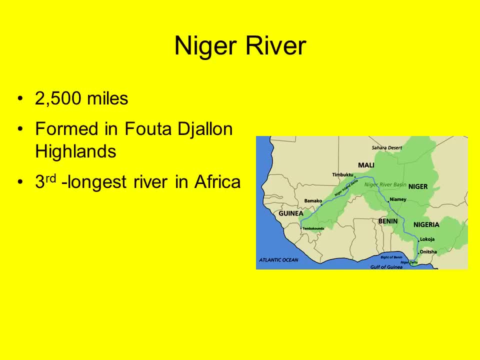 And likely referred to the inhabitants of the region. The Niger floods yearly. The flooding begins in about September, it peaks in November and finishes by May, And it, like many rivers in West Africa, has its source in the Futajalon Highlands region. 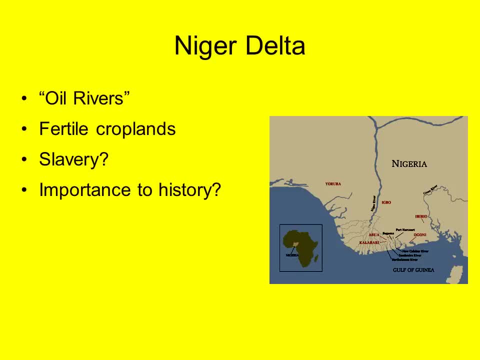 The Niger Delta. it's about 7.5% of Nigeria's land mass. Approximately 31 million people live in the Delta region. It has a significant amount of oil that's extracted from there- about 2 million barrels a day extracted in the Niger Delta. 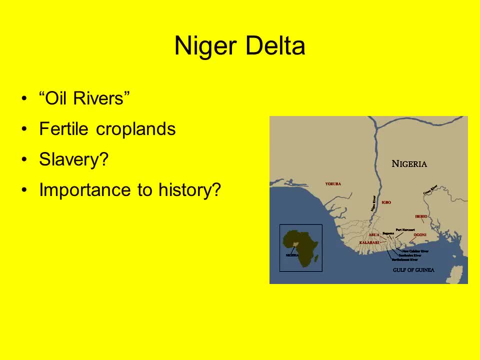 It's called the oil rivers for two reasons: not just for petroleum, but in the 19th century palm oil, or oil from palm trees, was highly prized by Europeans. It made an excellent machine lubricant. So there's a history of two different oil products that have been exported from this region. 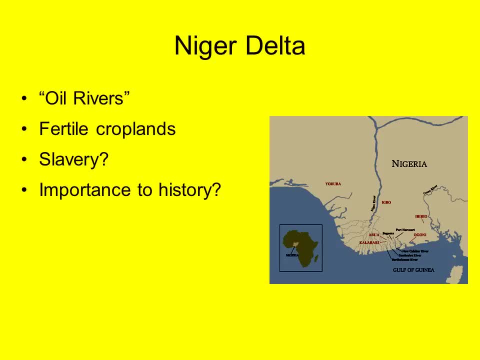 Many major ports for the transatlantic slave trade could be found in and around the Niger Delta. Because the Niger River extends so far into West Africa, it's more like a superhighway of sorts, or has been through history, and is navigable for long stretches. 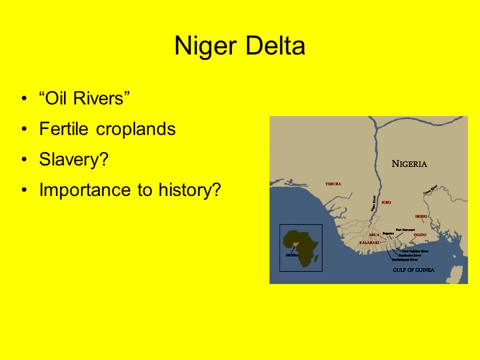 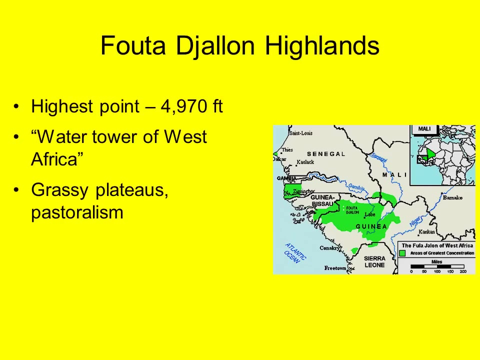 So it's not surprising that the transatlantic slave trade would be centered in part on the Niger River, And the control of this river and its delta has been the goal of many West African kingdoms. It has been extremely important in African history: The Futejelon Highlands, sometimes called the Water Tower of West Africa. 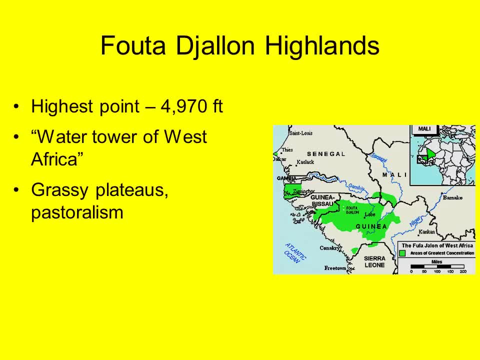 are the source of many West African rivers, including- well, we talked about- the Niger, but the Senegal and Gambia rivers also have their source here. Winds coming off the Atlantic Ocean hit the Futejelon Highlands. The water condensates collects on the ground. 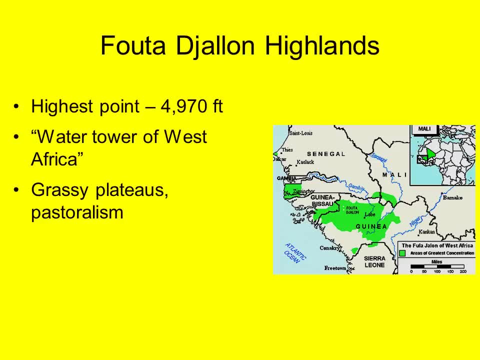 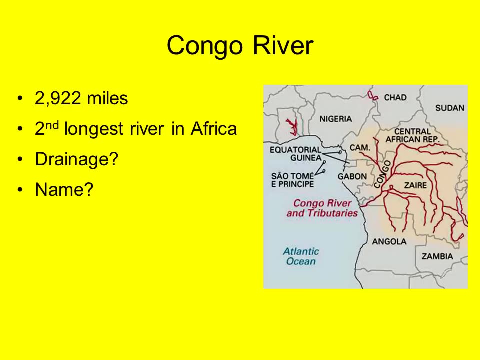 and rivers are formed. major rivers are formed in the Futejelon Highlands. This area has been a major center of Islam in West African history. The Congo River, at just a little under 3,000 miles in length, is the second longest river in Africa. 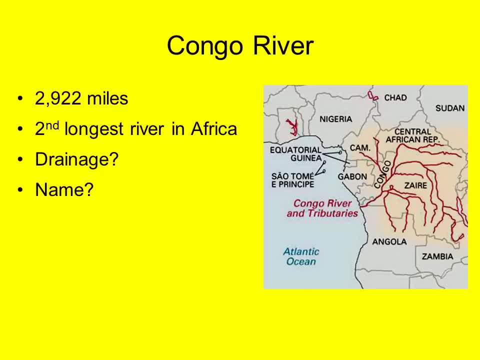 It's the ninth longest river in the world. In places it's up to 750 feet deep, and then in other places, because of waterfalls and rapids, it's very shallow. It is not navigable for long stretches due to this uneven nature of the depth of the river. 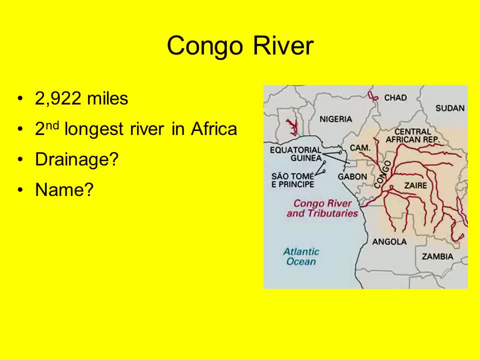 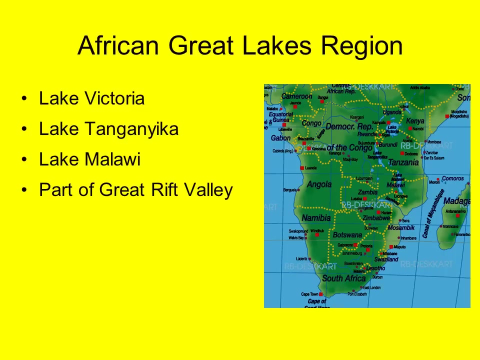 A significant portion of central and west Africa, and the drainage system goes into the Congo Basin. It is also the second largest in terms of water discharge in the world, after the Amazon Basin. The African Great Lakes region is important for a number of reasons, not the least of which is supply of fresh water for eastern and central Africa. 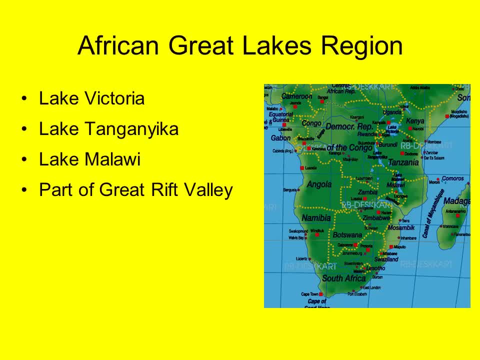 The biggest lakes are Lake Victoria, which is the second largest freshwater lake in the world in terms of surface area, Lake Tanganyika, which is the second largest lake in the world in terms of volume, and Lake Malawi. These are the largest of the Great Lakes. 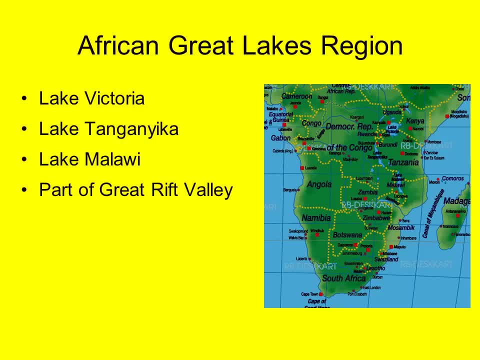 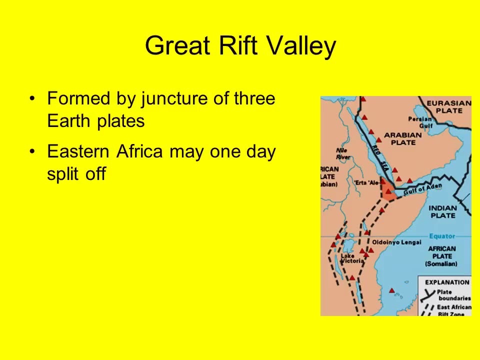 but there's hundreds of them really, some of them very small, and they're part of what is known as the Great Rift Valley of eastern Africa. The Great Rift Valley is an area of intense volcanic activity. It actually stretches from Syria all the way down to Mozambique in southern Africa. 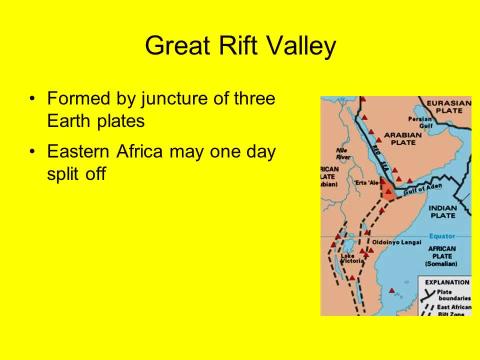 As you can see on the slide, three major tectonic plates collide in this region and the trend right now is that the eastern edge of Africa is going to split off from the rest of the continent. It's moving in different directions than the rest of the continent. 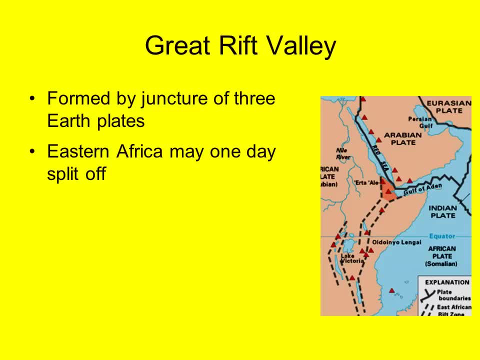 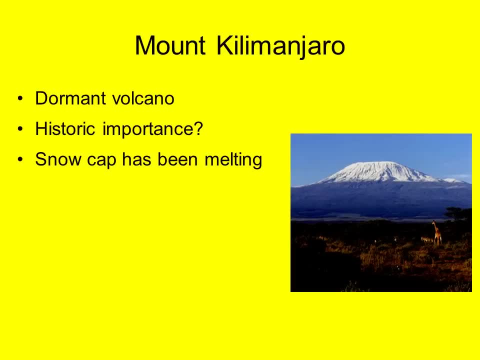 if you can study the arrows, the directional arrows. Mount Kilimanjaro, at 19,000 feet and some change- is the highest peak in Africa. The mountain is actually a dormant volcano and there were three cones at one point producing volcanic activity. 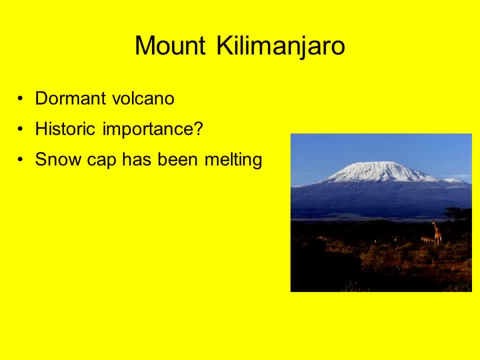 but two of them are extinct and one is dormant. the tallest one, Kibo. It would be several thousand feet taller had its top not blown off in an eruption several hundred thousand years ago. It's been important for several reasons in history. 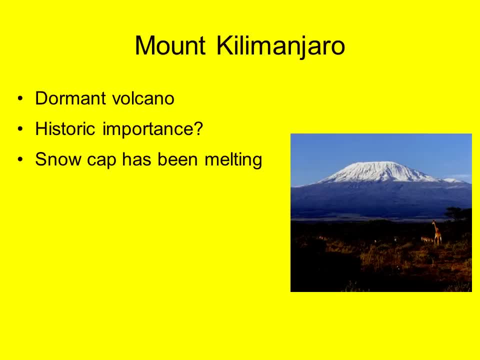 not the least of which is as an important source of water as the ice cap melts seasonally. It's also been a source of intense inquiry for Europeans when they heard about this very tall mountain in an area that was a very flat land around it. 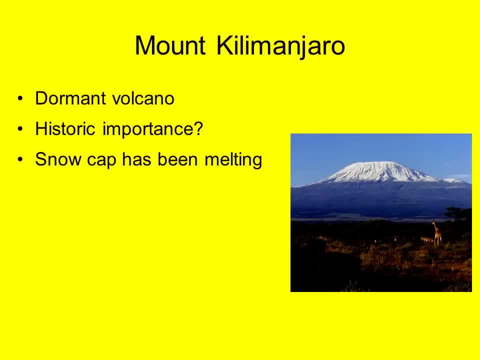 very fascinated by that, so they took some time before Europeans actually discovered it. discovered for them. It wasn't a discovery for people who had been living there and climbed it. That would be in the late 19th century. The snow cap, as I indicated on the slide, has been melting. 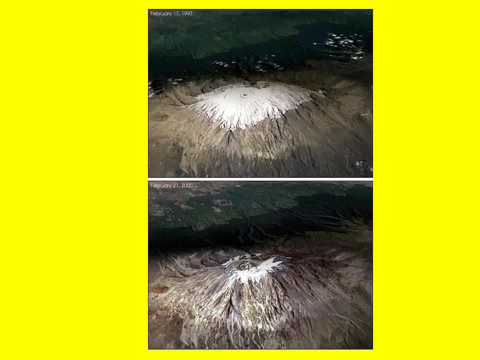 Over the past century, more than 80% of the ice cover on Mount Kilimanjaro has disappeared. Mount Kilimanjaro is expected to become completely ice-free by the year 2040 if current climatological conditions continue, And you can see in the images. 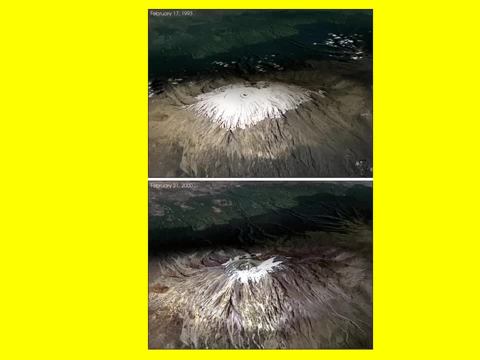 the upper image 1993, the lower image 2000.. And again, the debate, of course, is not whether this is occurring, but the extent to which human activity is responsible for this and how much is cyclical in nature. 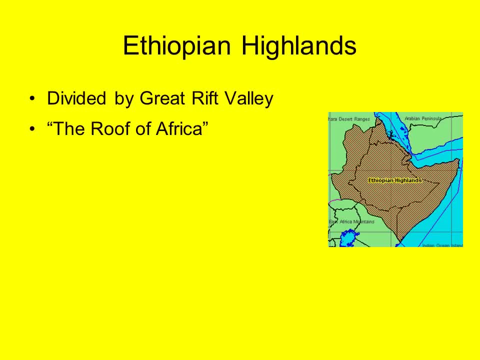 Finally, we'll end this lecture with a discussion of the Ethiopian highlands. There are peaks in this region up to 15,000 feet in height, sometimes called the roof of Africa because it's a large land mass that is highly elevated. 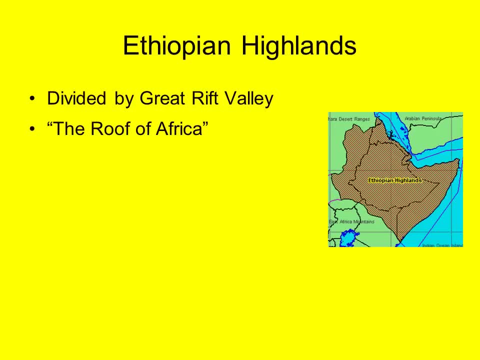 This region has a long history of human habitation in a number of significant civilizations. The Ethiopians have called this region home. One of the reasons why- and we'll get to Ethiopia in a later lecture- but one of the reasons why Ethiopia. 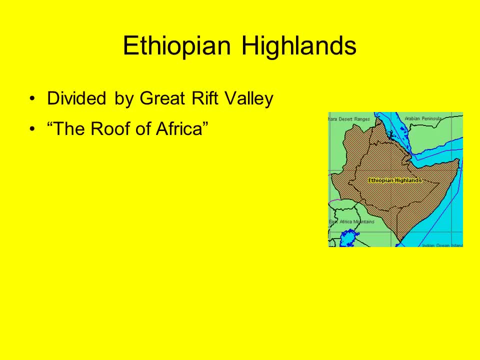 had such a continuous and stable civilization is because the Ethiopians, the people of Ethiopia, have been protected by living in this highland region, because it's very difficult to ascend. Even getting in there, you have to cross some difficult terrain. This brings to a close our brief overview of African geography.